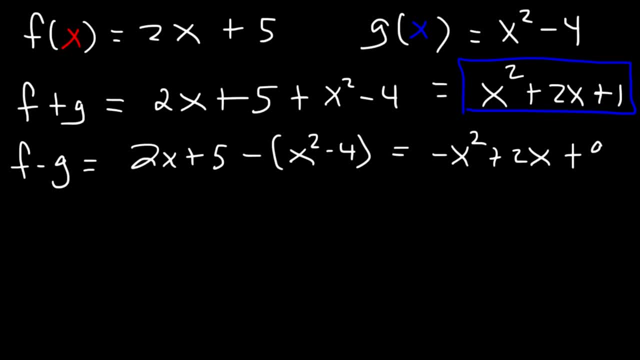 5 minus negative 4 is like 5 plus 4,, which is 9.. So that's equal to f minus g. Now what about f times g? This is just going to be 2x plus 5 times x, squared minus 4.. 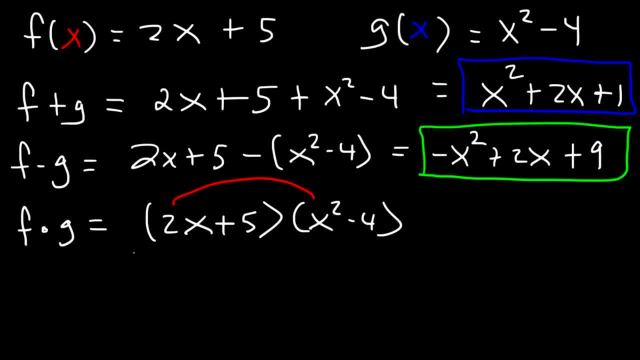 And we can go ahead and find that 2x times x squared, that's 2x cubed, and then 2x times negative 4,, that's negative 8x. And then we have 5 times x squared, that's 5x squared, and then 5 times negative 4, it's negative 20.. 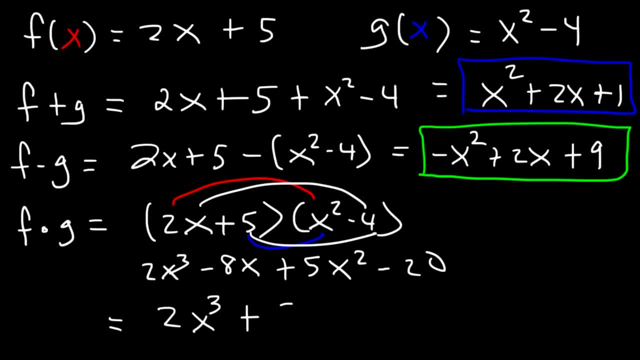 So in standard form, it's 2x cubed plus 5x squared, minus 8x minus 20.. Now, what is the domain of the three functions? Let's start with f plus g. What is the domain for that? Whenever you have a polynomial, be it a binomial, trinomial or many terms where you don't have any fractions, no radicals or logarithmic functions. 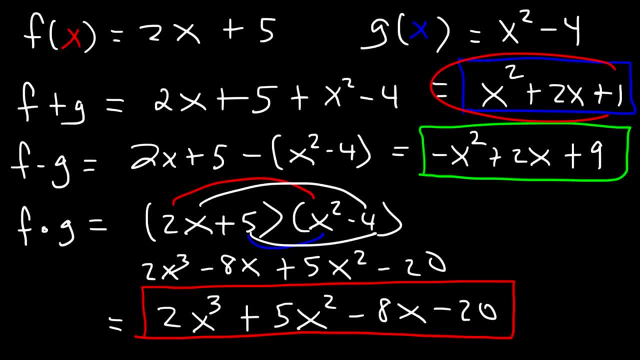 the domain will be all row numbers. There's no restrictions on the value of x in this expression. x can be anything. So for these three functions- f plus g, f minus g and f times g- we don't have any fractions or radicals. 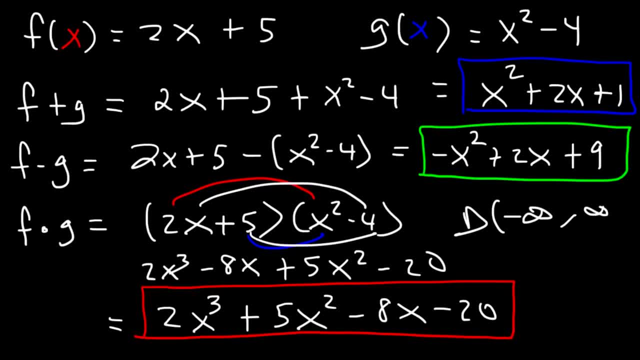 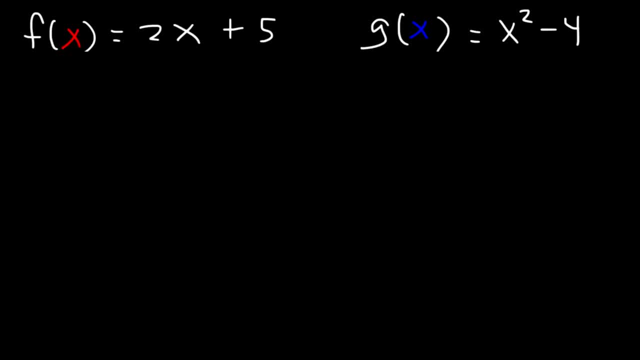 So the domain is all row numbers. It's negative infinity to infinity. Now what about f divided by g? What's the domain for this? f divided by g is simply 2x plus 5 divided by x squared minus 4.. Now that we have a fraction, the domain is restricted. 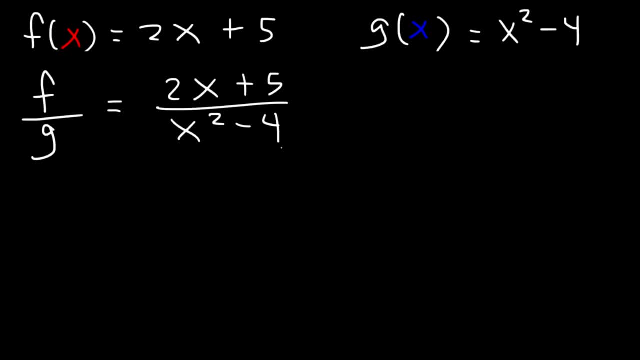 It's not all row numbers To find the domain. you want to find the x values that do not exist, The values that x cannot be. To do that, set the denominator equal to 0.. x squared minus 4 cannot be 0.. 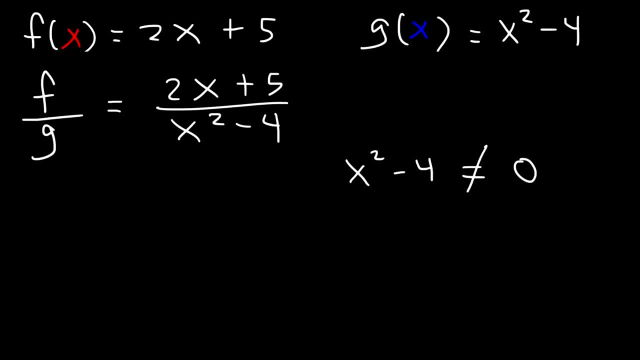 If it is, we're going to get a vertical asymptote, which means it's undefined at that point. Now we can factor x squared minus 4.. It's x plus 2 times x minus 2.. So therefore x cannot equal negative 2,. 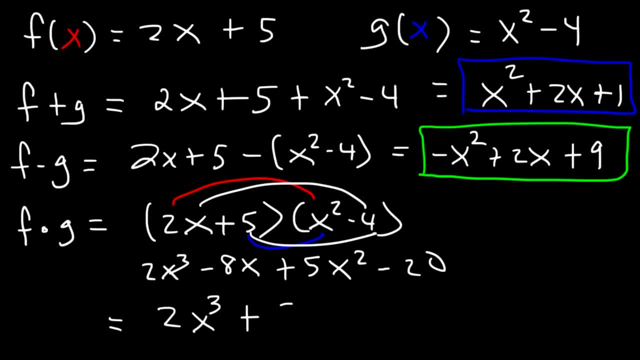 So in standard form, it's 2x cubed plus 5x squared, minus 8x minus 20.. Now, what is the domain of the three functions? Let's start with f plus g. What is the domain for that? Whenever you have a polynomial, be it a binomial, trinomial or many terms where you don't have any fractions, no radicals or logarithmic functions. 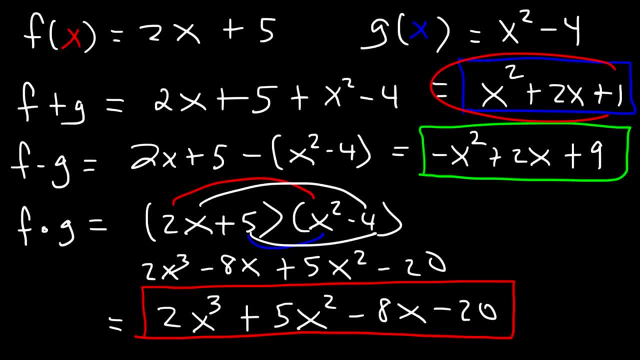 the domain will be all row numbers. There's no restrictions on the value of x in this expression. x can be anything. So for these three functions- f plus g, f minus g and f times g- we don't have any fractions or radicals. 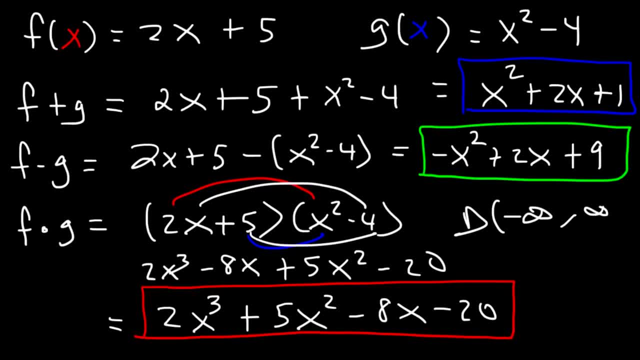 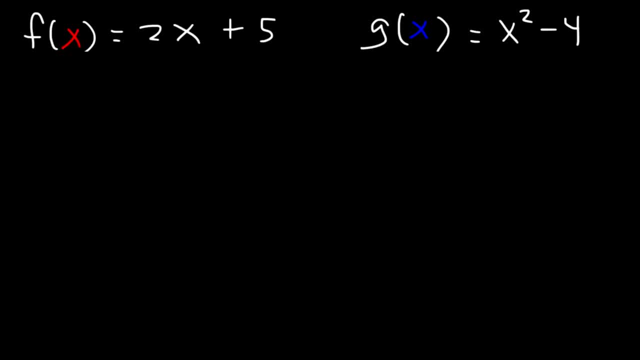 So the domain is all row numbers. It's negative infinity to infinity. Now what about f divided by g? What's the domain for this? f divided by g is simply 2x plus 5 divided by x squared minus 4.. Now that we have a fraction, the domain is restricted. 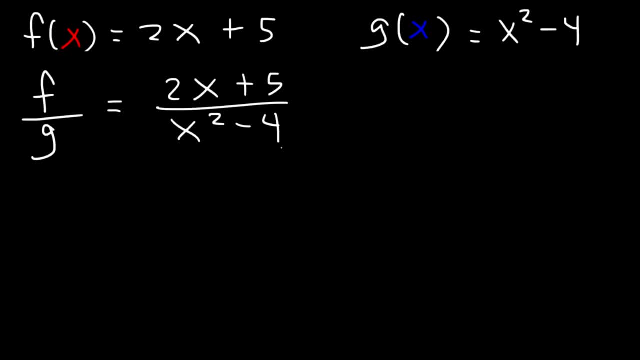 It's not all row numbers To find the domain. you want to find the x values that do not exist, The values that x cannot be. To do that, set the denominator equal to 0.. x squared minus 4 cannot be 0.. 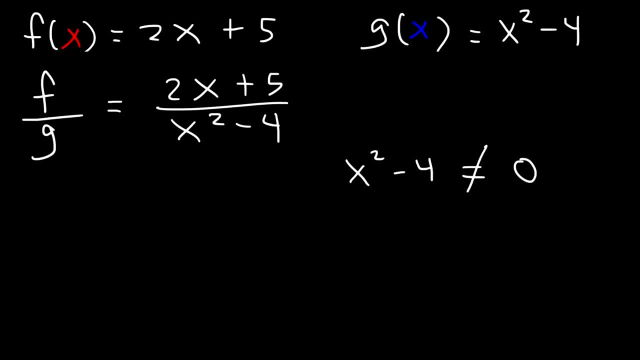 If it is, we're going to get a vertical asymptote, which means it's undefined at that point. Now we can factor x squared minus 4.. It's x plus 2 times x minus 2.. So therefore x cannot equal negative 2,. 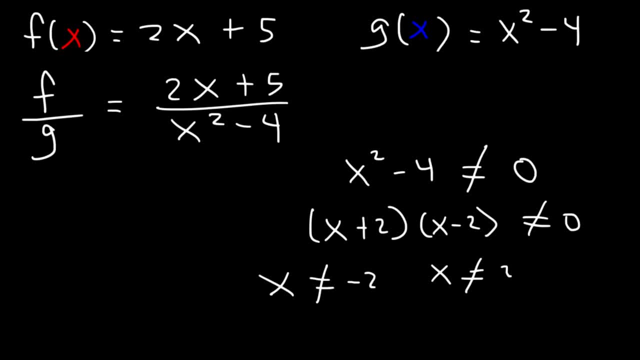 and it can't equal 2.. These are the vertical asymptotes, But they're also infinite discontinuities. There's no, we can't plug in negative 2 for x. The function will be undefined. Anytime you have a 0 on the bottom, it's undefined. 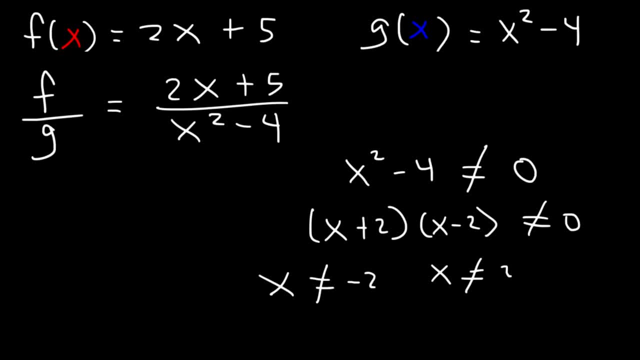 and it can't equal 2.. These are the vertical asymptotes, But they're also infinite discontinuities. There's no, we can't plug in negative 2 for x. The function will be undefined. Anytime you have a 0 on the bottom, it's undefined. 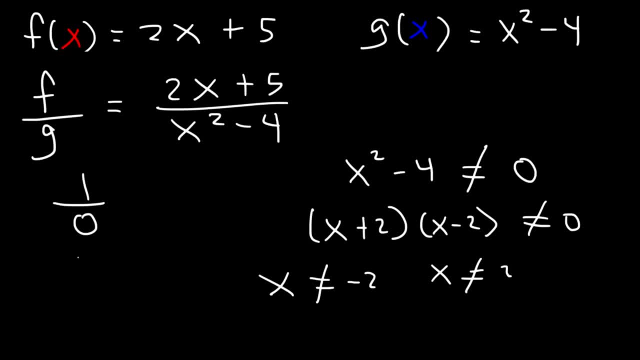 So how can we write the domain using interval notation if x cannot equal negative 2 or 2? It's going to be from negative infinity to negative 2, union negative 2, negative 2.. So we're going to write the domain using interval notation. 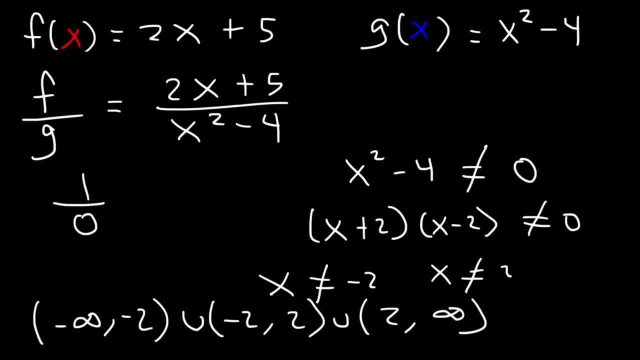 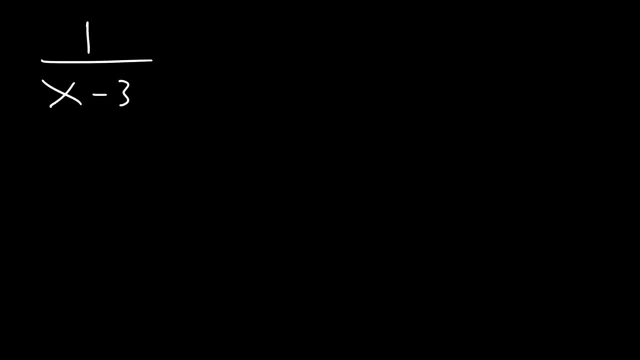 2 to 2, union 2 to infinity. So here's another example. Let's say, if we have the function 1 over x minus 3.. x minus 3, the denominator cannot be 0. So x cannot be 3.. 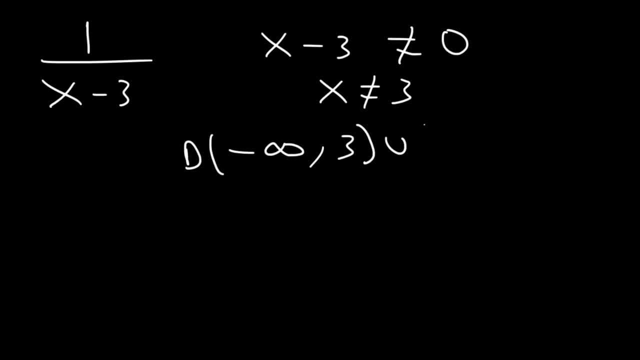 Therefore the domain is everything except 3.. That's how you'll write it. Let's say: if we have this, x cannot equal 4, and it can't equal negative 3. Just change the sign If you set x minus 4 to 0,. 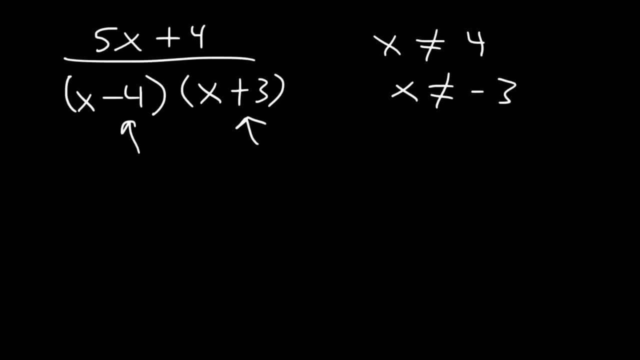 x, you'll get 4 for x. Now to write the domain, it's going to be negative. infinity to negative 3.. Negative 3 comes before 4. Union. negative 3 to 4. Union. 4 to infinity. 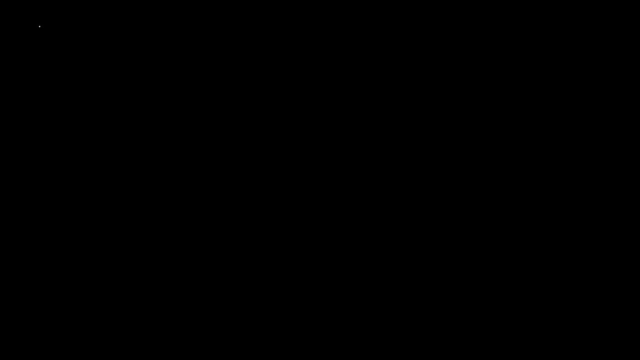 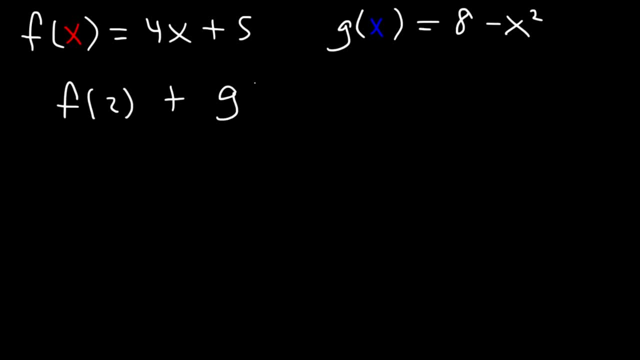 What is f of 2 plus g of 3?? To find f of 2, we need to replace f of 2 with x with 2 in the equation 4x plus 5.. So that's 4 times 2 plus 5.. 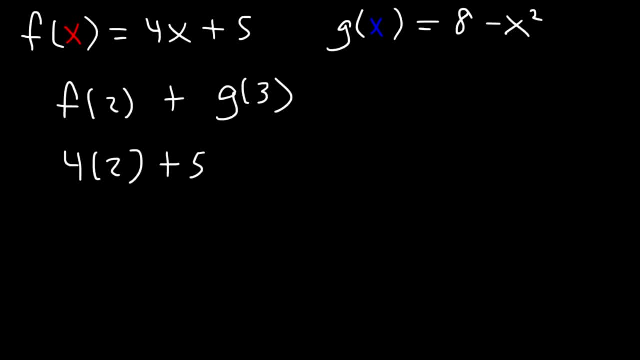 And that is a terrible looking 2.. To find g of 3, we need to plug it into that equation. So it's plus 8 minus 3 squared, And then let's add: 4 times 2 is 8,. 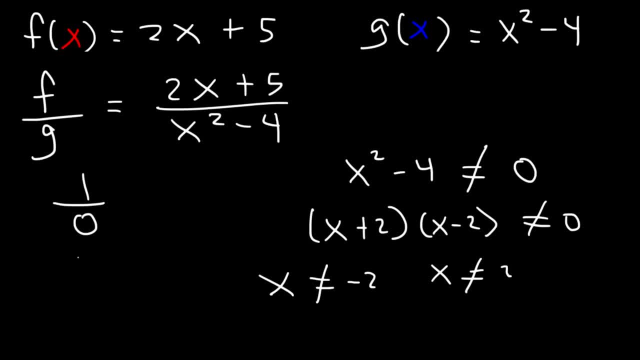 So how can we write the domain using interval notation if x cannot equal negative 2 or 2? It's going to be from negative infinity to negative 2, union negative 2 to 2, union 2 to infinity. So here's another example. 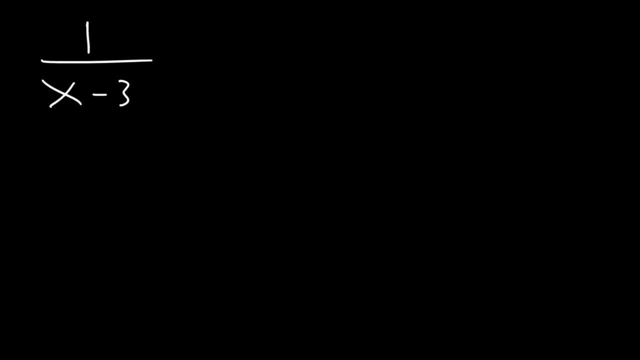 Let's say, if we have the function 1 over x minus 3.. x minus 3, the denominator cannot be 0. So x cannot be 3.. Therefore, the domain is everything except 3.. That's how you'll write it. 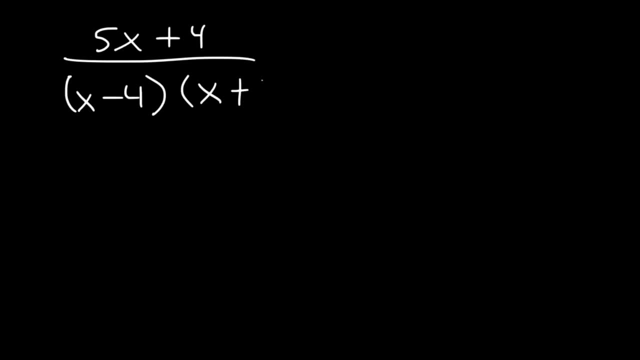 Let's say, if we have this, x cannot equal 4, and it can't equal negative 3.. Just change the sign. If you set x minus 4 to 0, x, you'll get 4 for x. Now to write the domain: 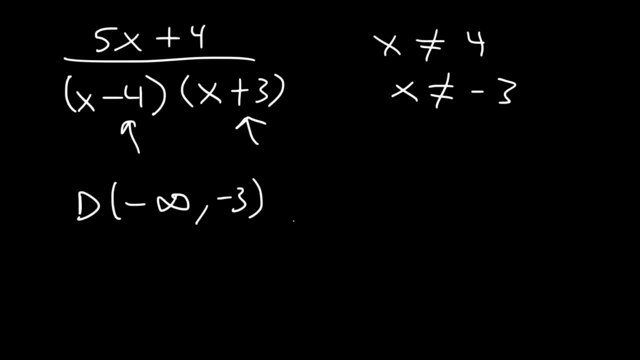 it's going to be negative infinity to negative 3. Negative 3 comes before 4. Union. negative 3 to 4. Union. 4 to 4. Union. 4 to 4.. 4 to 4.. 4 to 4.. 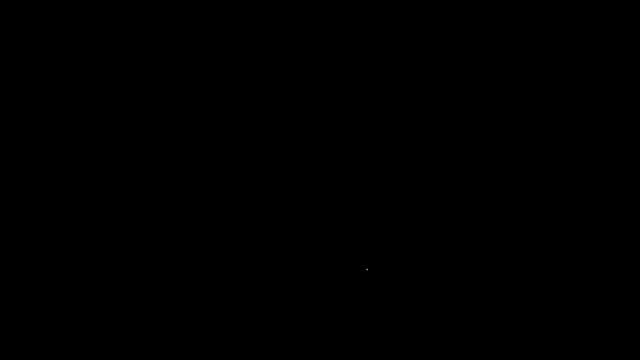 4 to infinity. So that's the domain for this function. So let's say that f of x is equal to 4x plus 5, and g of x, let's say it's equal to 8 minus x. squared, What is f of 2 plus g of 3?? 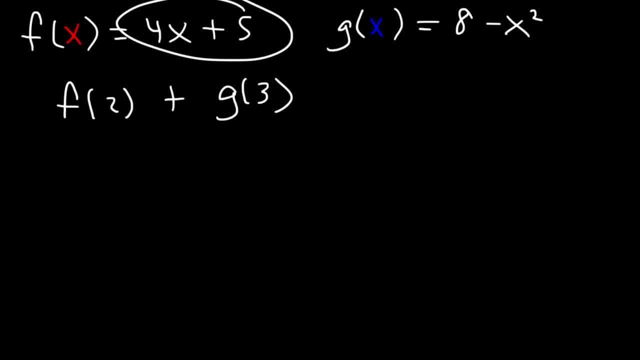 Define f of 2.. Define f of 2.. We need to replace x with 2 in the equation 4x plus 5. So that's 4 times 2 plus 5. And that is a terrible looking 2.. 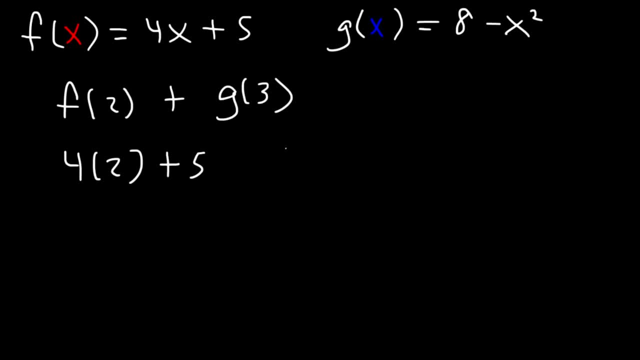 To find g of 3, we need to plug it into that equation. So it's plus 8 minus 3 squared, And then let's add 4 times 2 is 8, and 3 squared is 9.. 8 plus 5 is 13.. 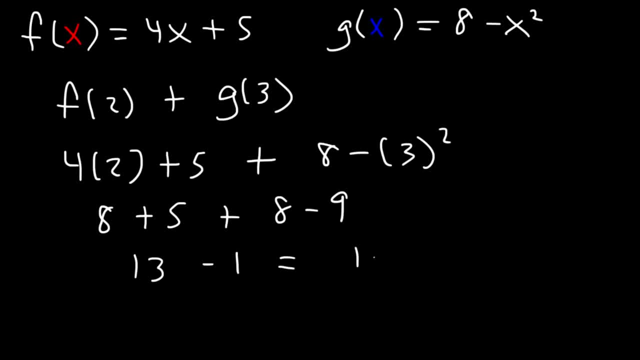 8 minus 9 is negative 1.. 13 minus 1 is 12.. So that's the value of f of 2 plus g of 3. You just find the two values and you add them. Let's try another example. 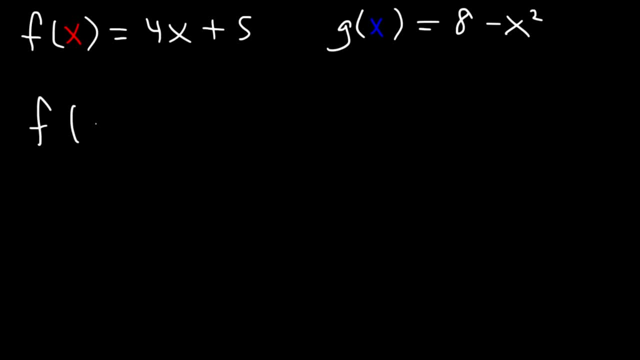 So what is f of negative 2 multiplied by g of 2?? So let's do it separately. Let's find f of negative 2 first Using this formula. So it's going to be 4 times negative 2 plus 5..